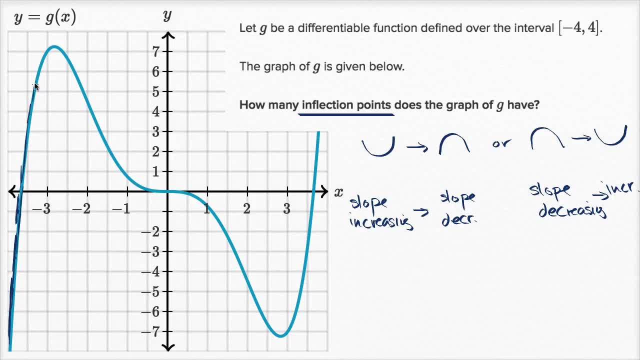 decreasing, decreasing. slope is decreasing, decreasing even more, it's even more, and then it's actually going to zero. our slope is zero, and then it becomes negative. So our slope is still decreasing, And then it's becoming more and more and more negative. 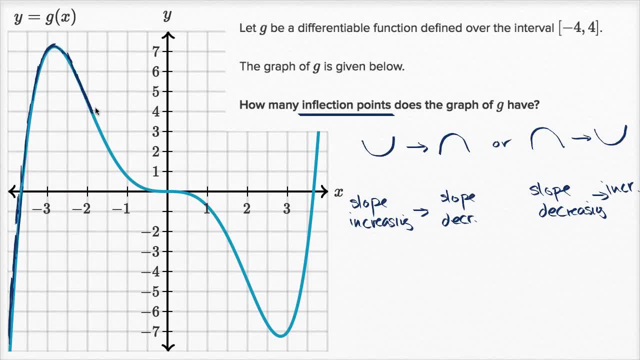 and then, right around here, it looks like it starts becoming less negative or it starts increasing. So our slope is increasing, increasing. it's just becoming less and less negative And then it's going close to zero, approaching zero. It looks like our slope is zero right over here. 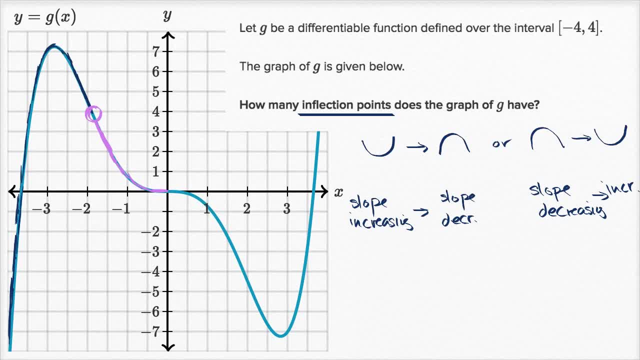 But then it looks like, right over there, our slope begins decreasing again, So it looks like our slope is decreasing again. So it looks like our slope is decreasing. It's becoming more and more and more and more negative, And so it looks like something interesting. 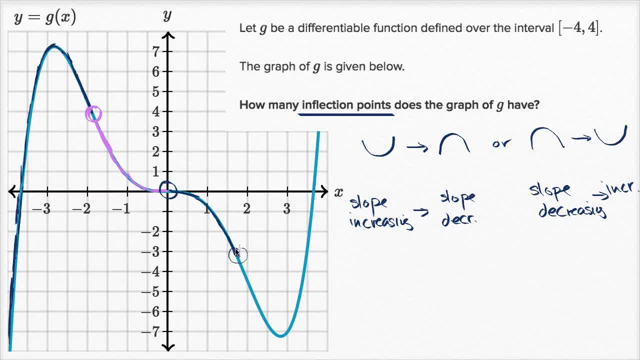 happened right over there. We had a transition point And then right around here it looks like the slope starts increasing again. So it looks like the slope starts increasing. It's negative, but it's becoming less and less and less negative and then it becomes zero. 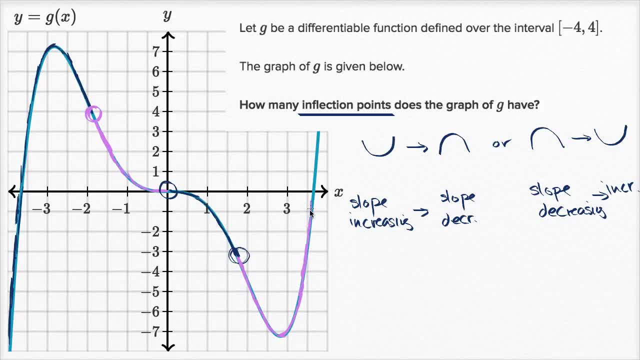 and then it becomes positive and then more and more and more and more positive. So inflection points are where we go from slope increasing to slope decreasing, So concave upwards to concave downwards, And so slope increasing was here- to slope decreasing. so this was an inflection point. 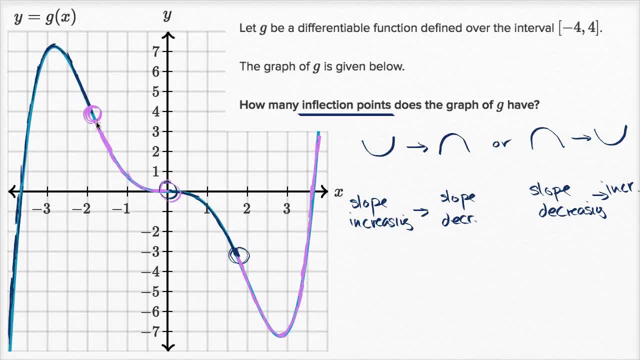 And also from slope decreasing to slope increasing. So that's slope decreasing to slope increasing And this is also slope decreasing to slope increasing. So how many inflection points does the graph of G have that we can see that we've on this graph? 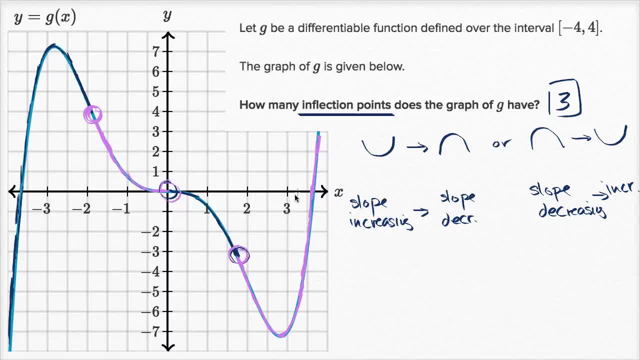 Well, it has three over the interval. that at least we can see.